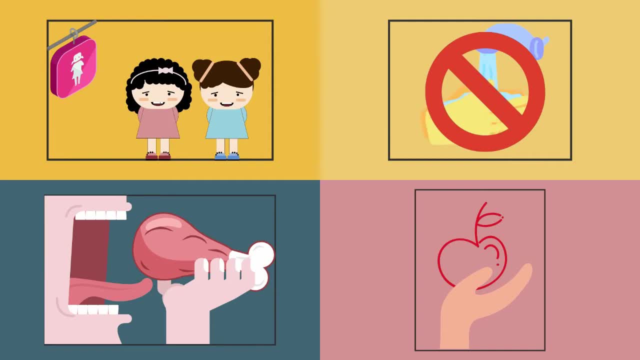 him to protective the women who were engaged with him. many times, Each one of his friends and family took papers He decided to sign to my parents'осcapes for plastics. They also sat down and read in the, For example: it is important for us to know how to handle and keep our food safe and clean. 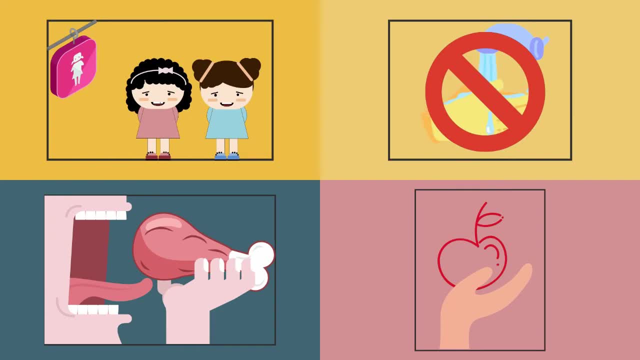 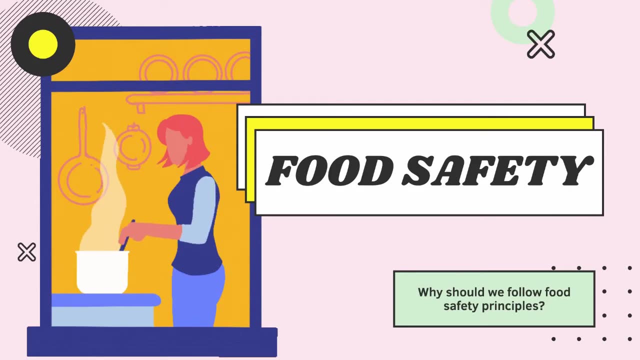 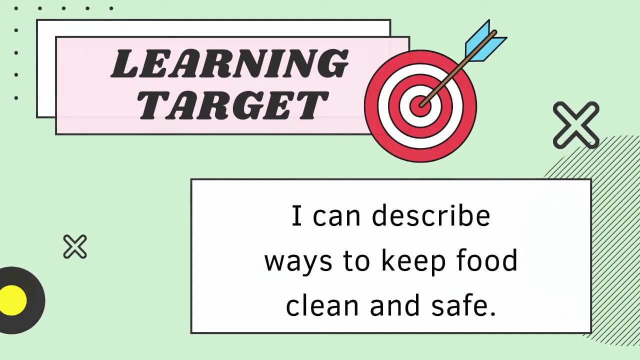 By having clean and safe food, we can avoid any foodborne diseases, such as diarrhea. Now let's talk about food safety. Here is our learning target. Read with me. I can describe ways to keep food clean and safe. Food gives us energy and makes the body strong and healthy. 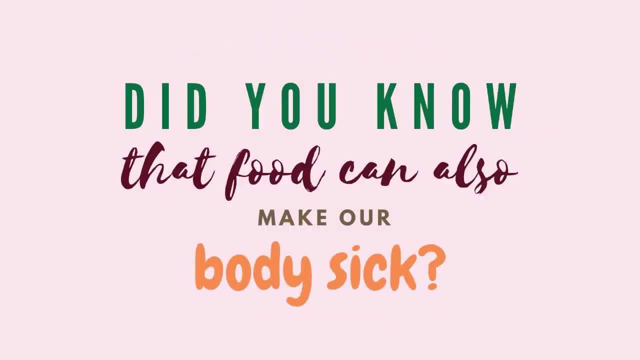 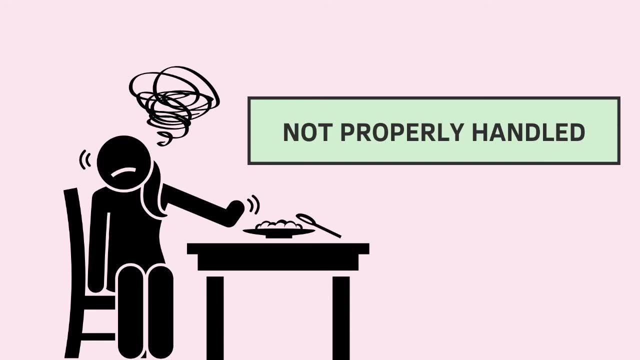 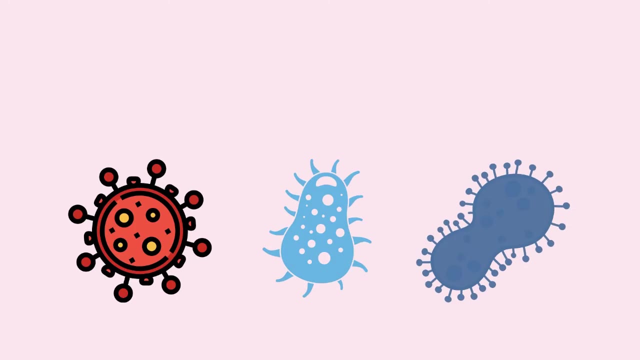 But did you know that food can also make our body sick, That is, if the food eaten are not safe and not properly handled or not properly prepared. There are diseases caused by eating unclean and unsafe foods. The good thing is that these diseases can be prevented. 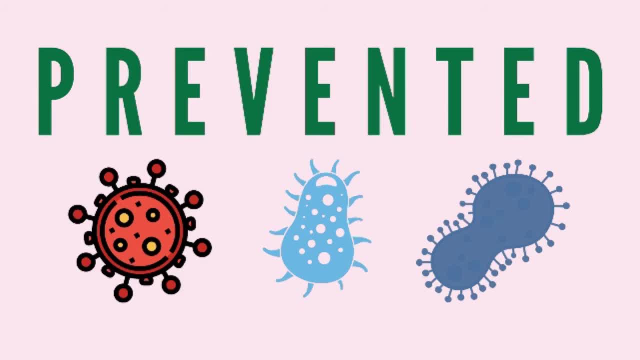 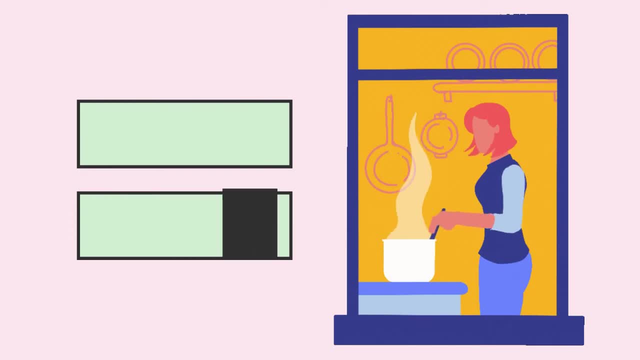 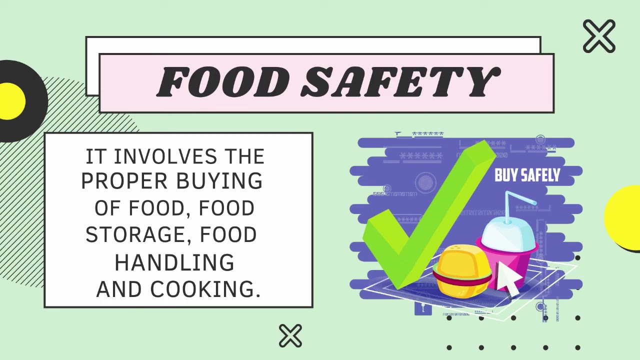 Since these diseases are caused by eating unclean and unsafe foods, then it is important to keep our food clean and safe. This is called food safety. Food safety involves the proper buying of food, food storage, food handling and cooking. This includes water, because it is also very important. 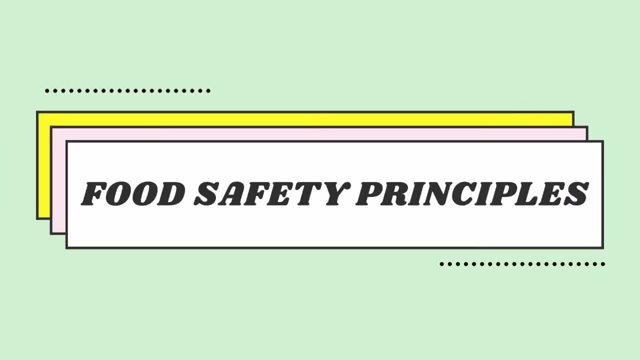 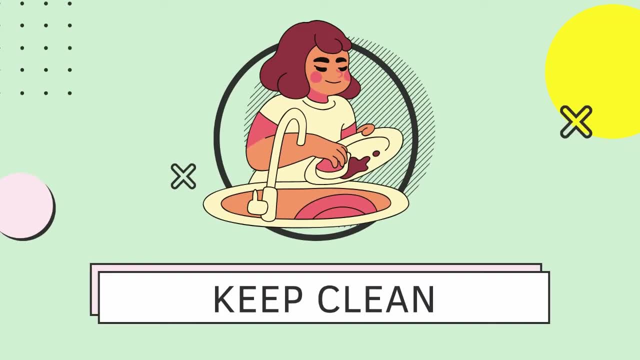 To guide us in making sure that food remains clean and safe. here are the food safety principles: Keep clean, Always, practice good personal hygiene and observe cleanliness in your surroundings. Doing both every day will lessen your risk of food hazards When you need to buy food outside the house, observe if the food handlers are healthy and 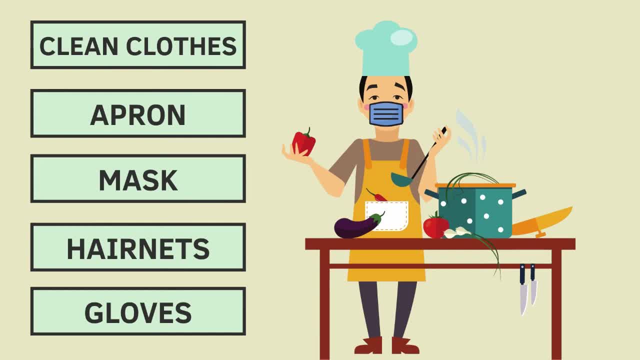 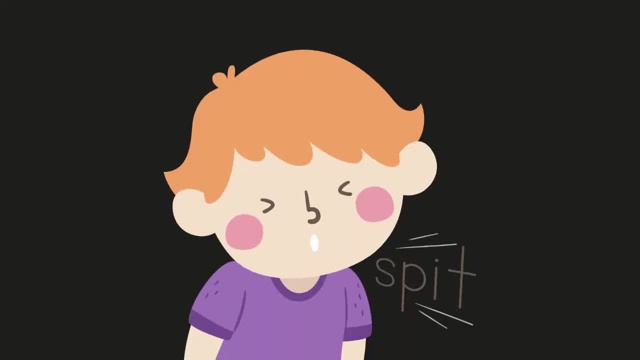 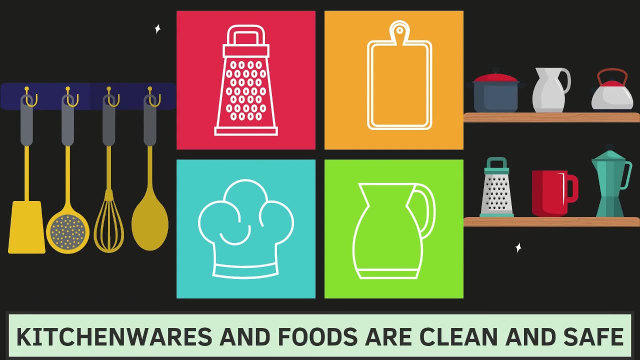 are wearing clean clothing like washable aprons, masks, hairnets and plastic gloves. Avoid unhygienic practices like spitting anywhere or blowing or picking your nose Even though the kitchen looks orderly. make sure the utensils, cutting boards, table. 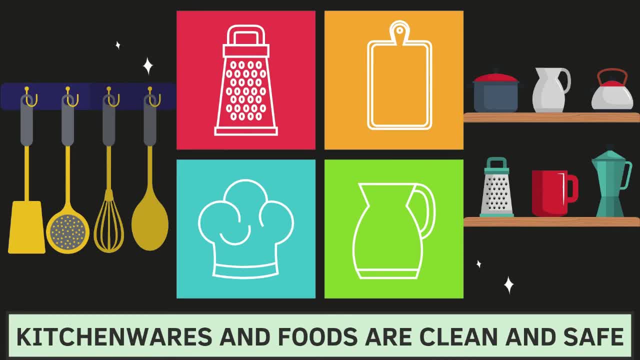 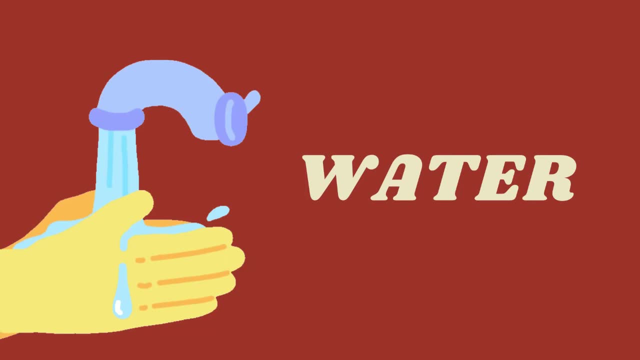 kitchen countertops and floors are clean before and after using them. Check also if your utensils, food and water containers and your lunchbox are clean. Wash your hands properly before preparing and eating food. When you wash your hands, do it with warm water and liquid soap.